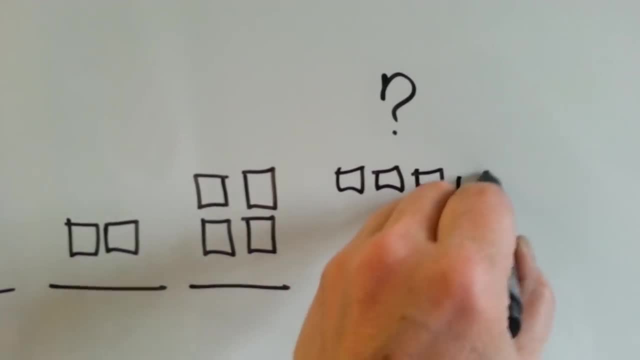 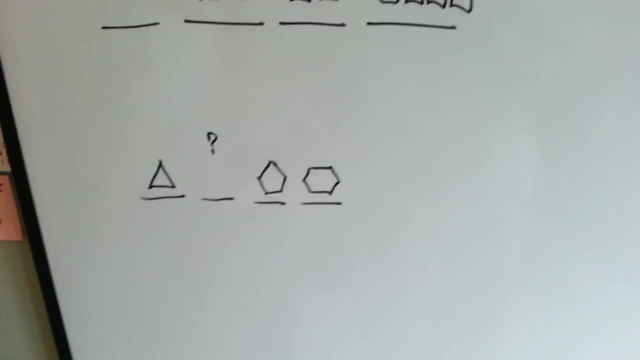 We'd put in eight of them, wouldn't we? That's what's missing. Should be eight squares. How about here? Can you see what these shapes are doing? What shape should go here, Here, Here, Here, Here, Here? 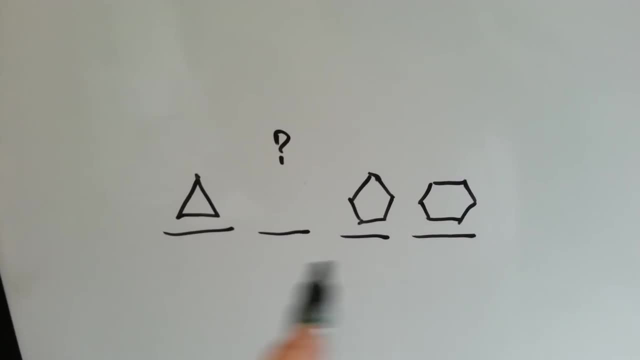 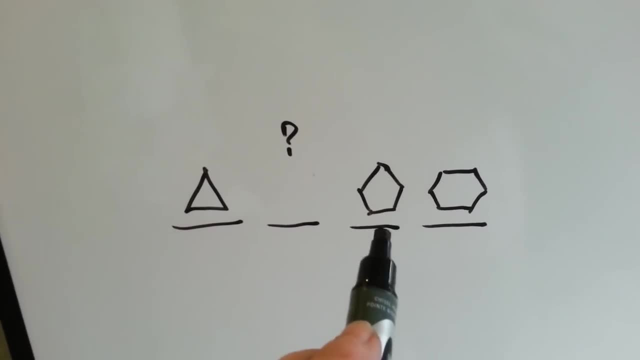 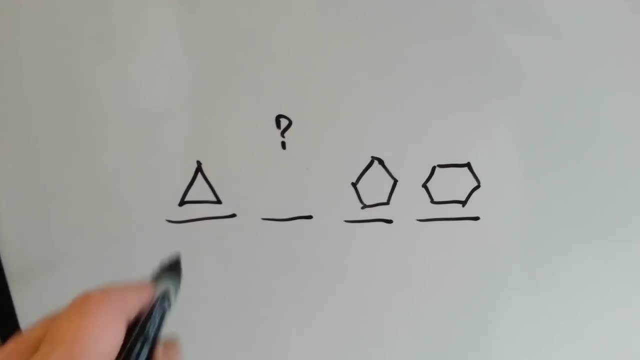 and this one's got one, two, three, four, five, six sides. Well, if this one's got three sides and this one's got five sides and this one's got six sides, guess what goes there? Did you figure it out? 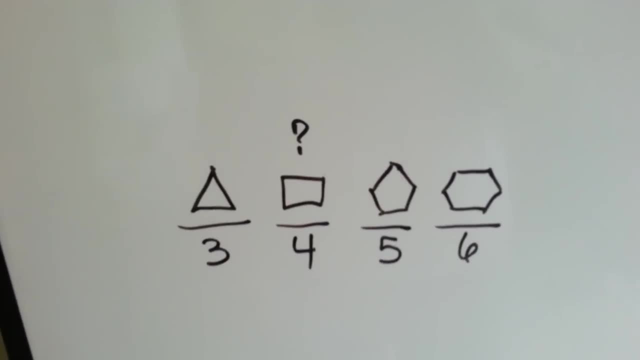 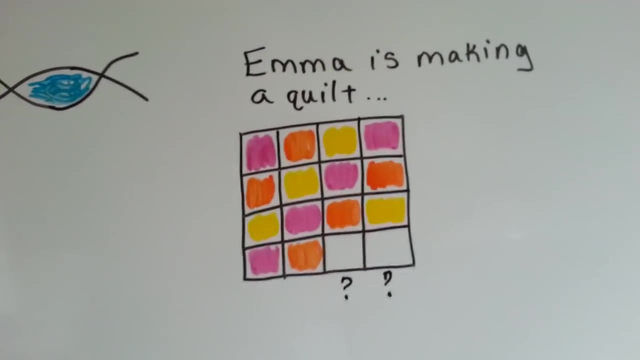 Something with four sides right, A rectangle or a square or a rhombus or a parallelogram, anything that would have four sides right. Okay, what if Emma was making a quilt and she ran out of fabric and she needed to go buy fabric? 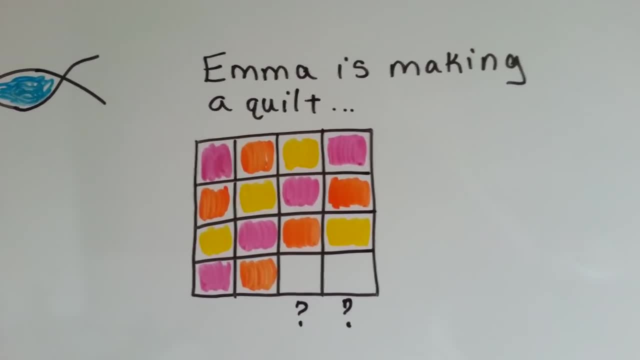 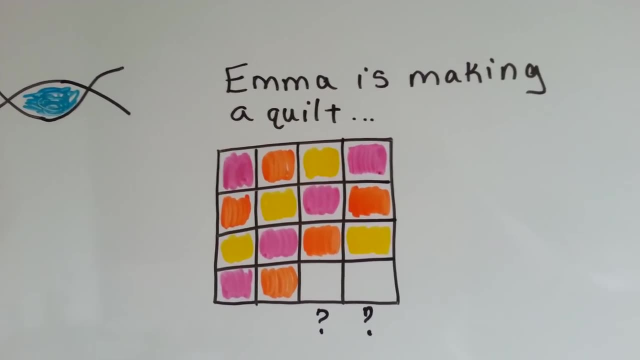 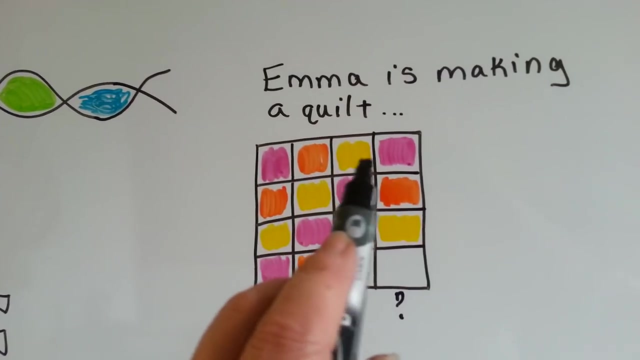 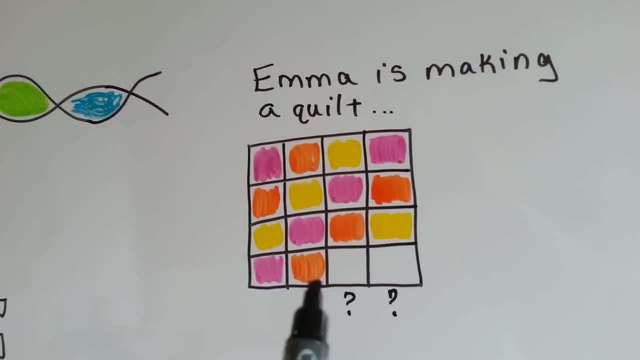 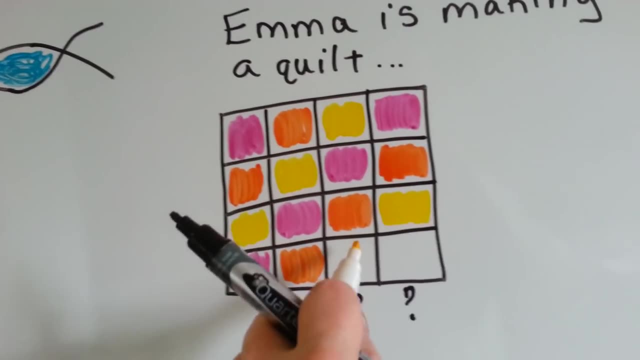 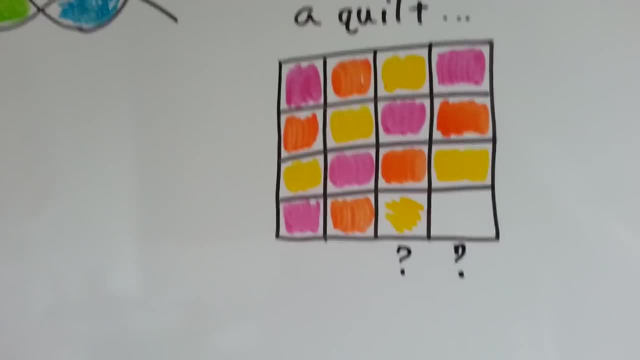 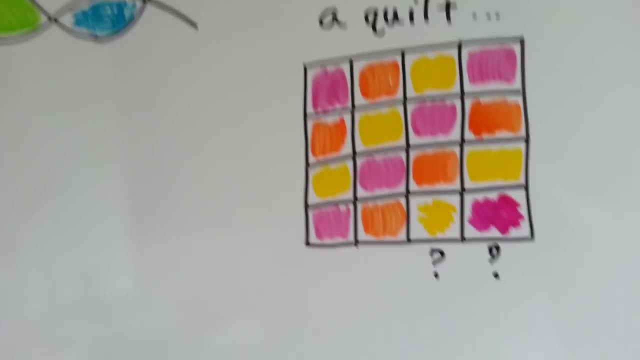 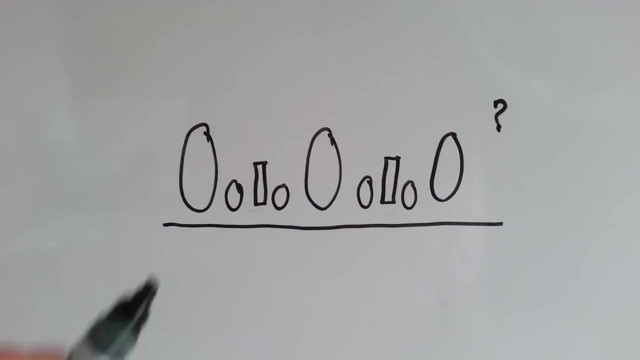 What comes after the yellow Should be a pink one. If you said pink one, you got it right. So we use the ones before it to help us figure out what comes next. We use the pattern. see How, about here? What shape should come next? 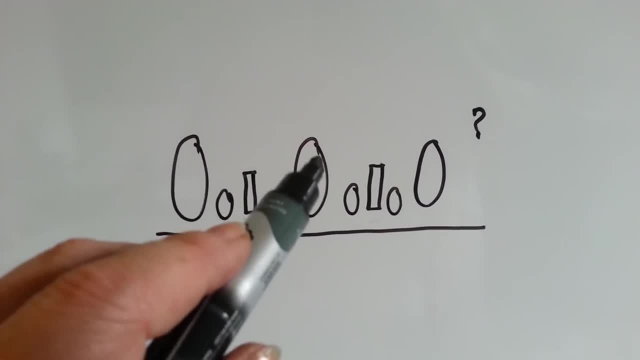 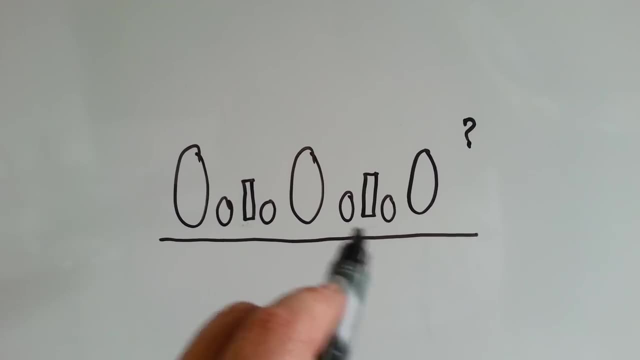